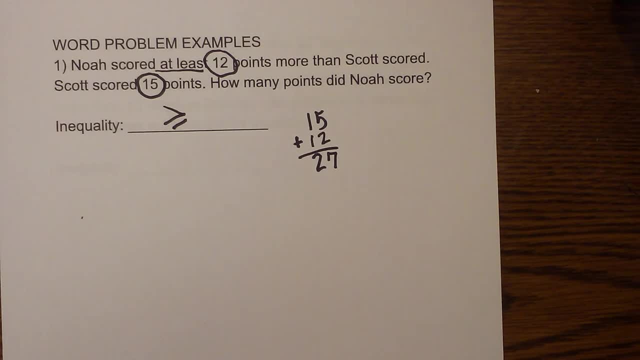 And so you want to know how many points did Noah score? And Noah scored at least 12 more than Scott, So there's some wiggle room there. So next, what it says is: we're going to write an x first and we're going to write the inverse. 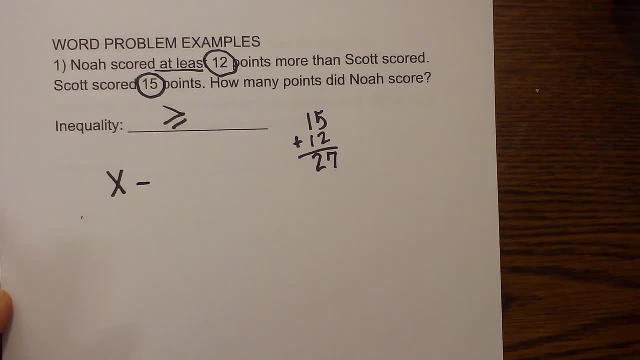 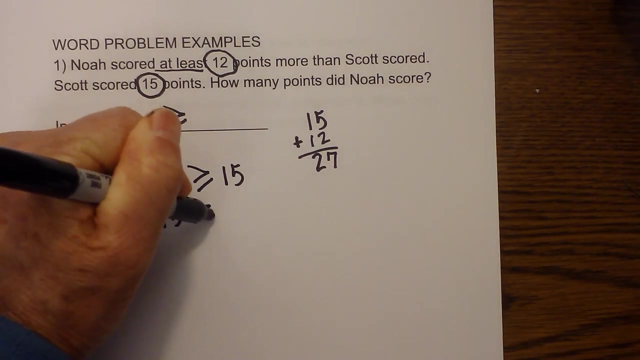 operation, which is subtraction. Then we are going to write the numbers, And I'm going to write 12 first, plus the inequality sign that we came up with, and then the other number. So that is one solution. Or we could write 12 minus 15, greater than or equal, put the inequality sign and then 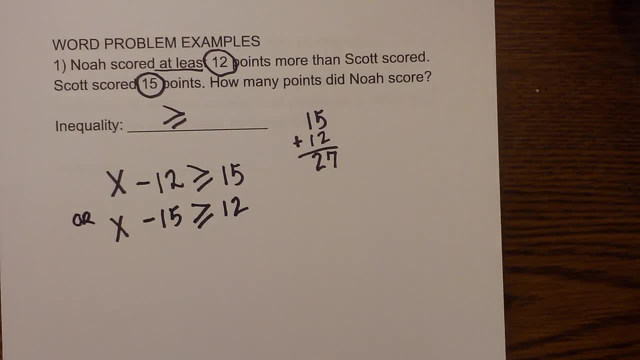 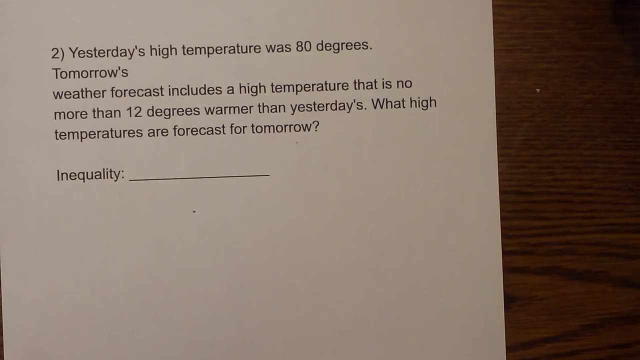 12.. So either one of those. So those are your solutions. Let's work one more. It says yesterday's high temperature was 80 degrees. Tomorrow's weather forecast includes a high temperature that is no more than 12 degrees. What high temperatures are forecast for tomorrow? 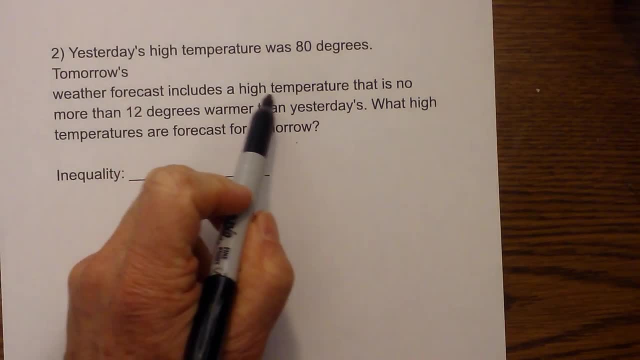 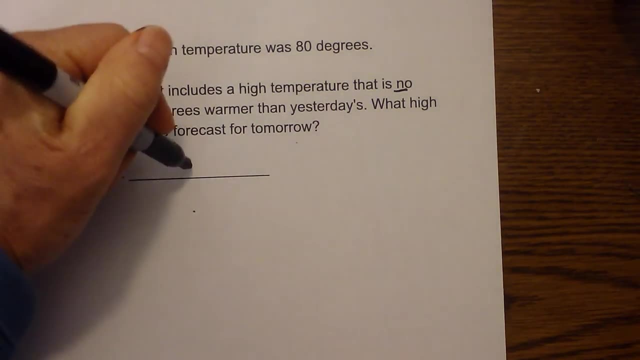 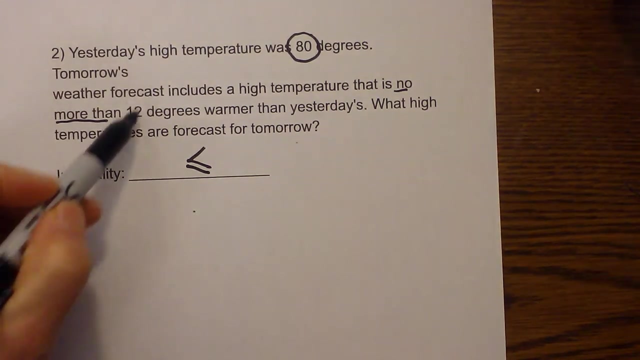 Let's first identify the inequality. It says includes a high temperature. that is no more than, No more than And no more than is going to be less than or equal to, And next We'll circle our numbers. We have 80 and 12.. 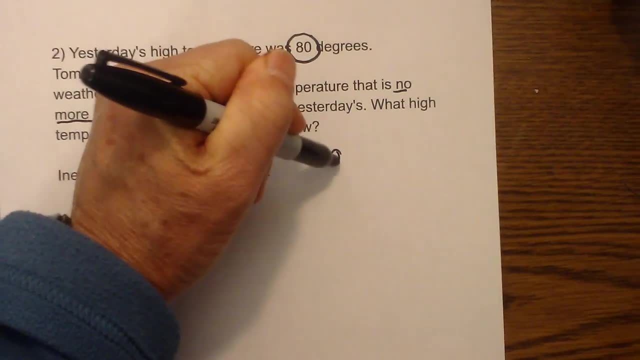 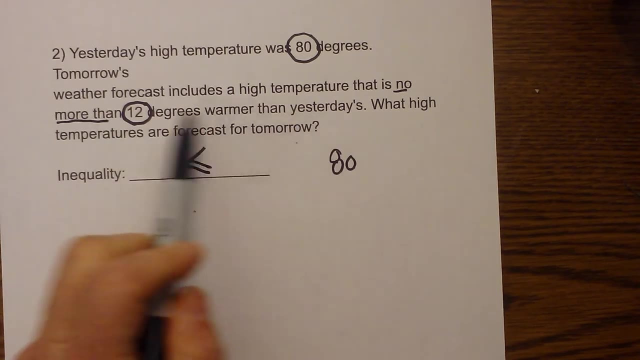 Now we need to find a solution. It says: let's begin. We have a high temperature of 80 and that it is no more than 12 degrees warmer. So it's going to be at least 12 degrees warmer. So I'm going to add 12.. 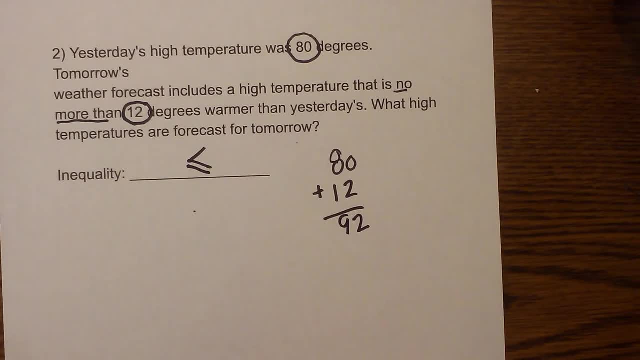 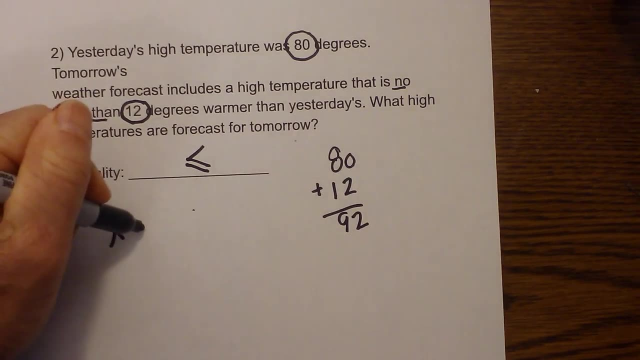 And that will give you a solution of 92.. So now I need to go ahead and write this out. I'm going to start with x, Put in the inverse Inverse operation, which is addition. So I'm going to use subtraction. 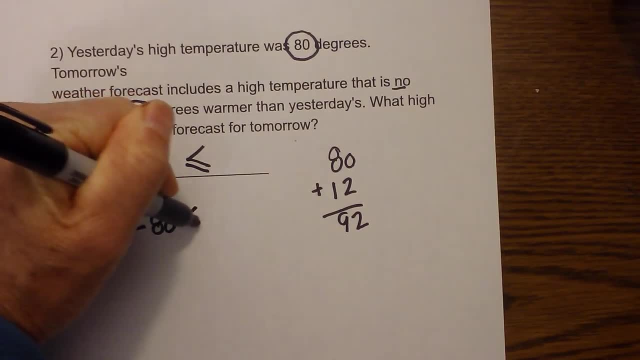 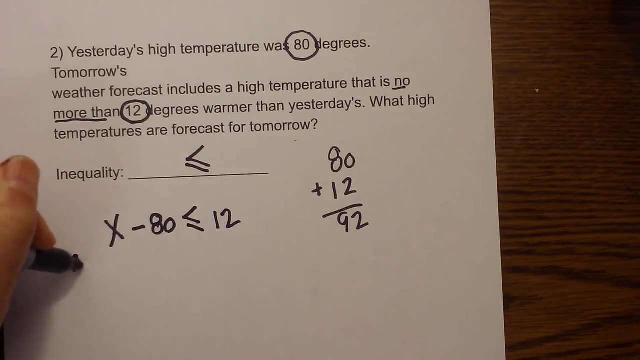 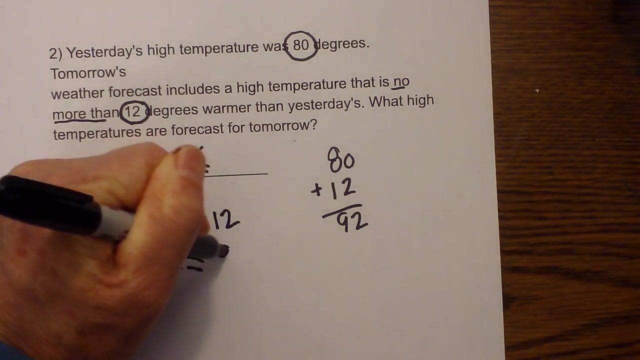 Use the numbers. I'll write 80 first, Put in the inequality sign And then write the other number on the other side And then OR do x inverse operation, minus 12, less than or equal to 80. I hope that helps in solving inequality word problems. 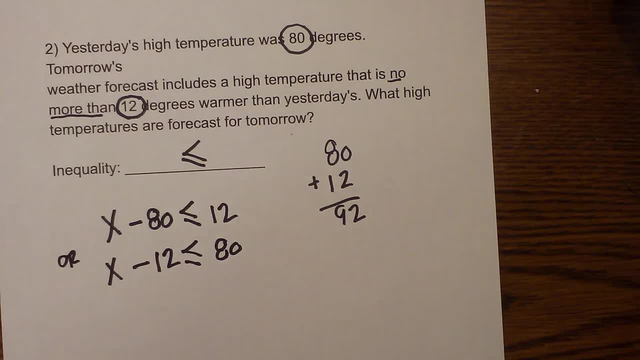 Just follow the steps and MooMoo Math and Science uploads a new math and science video every day. Please subscribe and share.